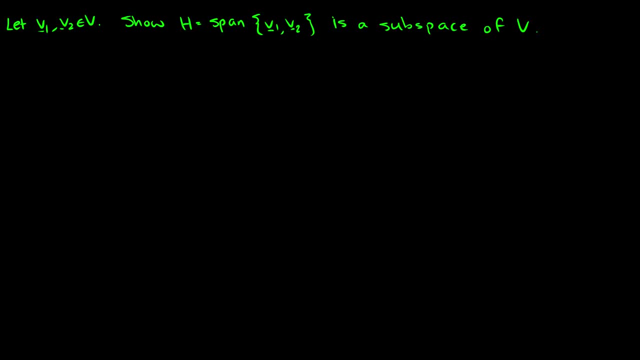 Okay, here is a little bit of a trickier question. So let V1 and V2 be in V and we want to show that H- which is the span of V1 and V2, is a subspace of V. So what we have to do is we have to check. okay, number 1 is 0 in the subspace. 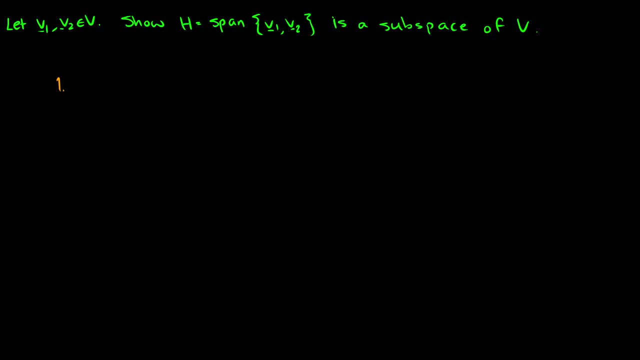 So that's our first step. So if we take 0,, which is equal to 0V1 plus 0V2, then of course this is going to be in our subspace H. So the first criteria is good. 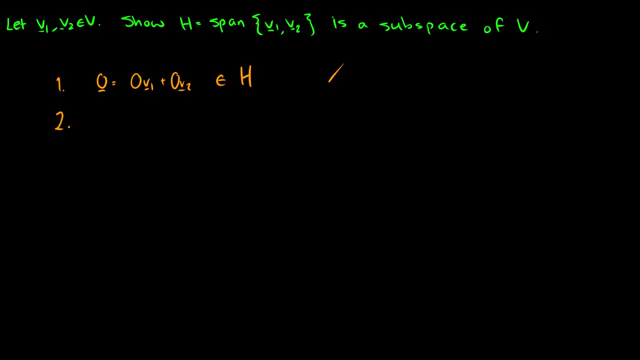 For the second criteria, we need to define V1 and V2.. So we're going to take V1 equal to S1. I shouldn't do this S1. I shouldn't label this V1. I'm going to label this U and we're going to have this S1V1 plus S2V2.. 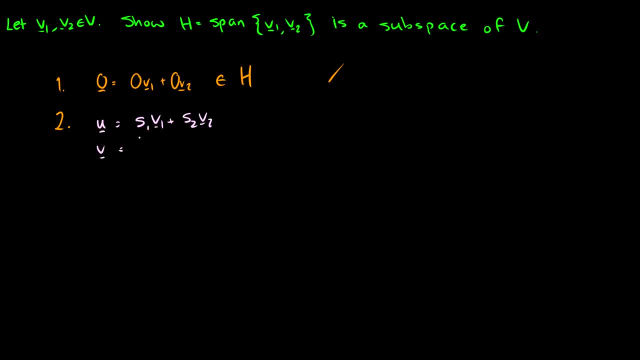 And then we're going to have a vector V which is equal to T1V1 plus T2V2.. Okay, so we have U, we have V. We're going to say that these are in H, So we have to show that U plus V is in H. 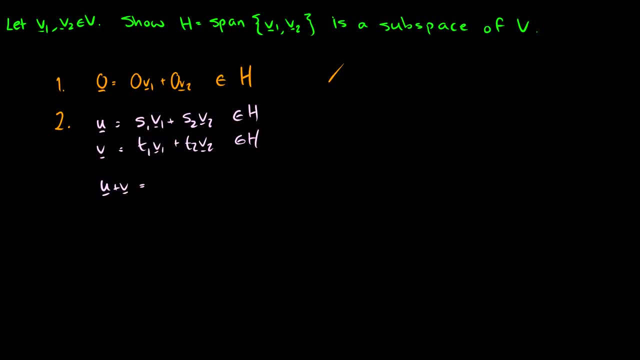 So U plus V is going to equal- well, we can gather the like terms here. So we have S1 plus T1 times V1, plus S2 plus T2 times V2.. And we know this is going to be in H, because this vector here is in the span. 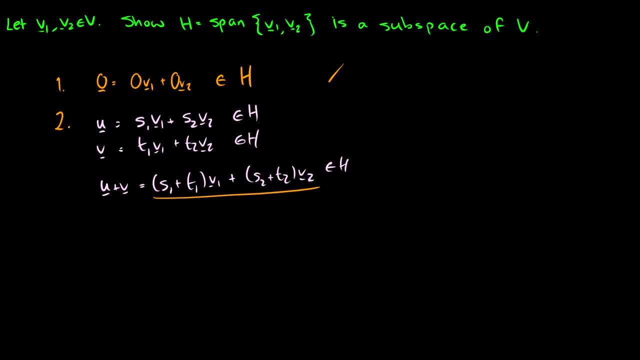 And our H is the span. Therefore U plus V is going to be in the subspace. So the second condition holds. The third condition: we need to check to see that C times any vector for any scalar is going to be in the subspace. 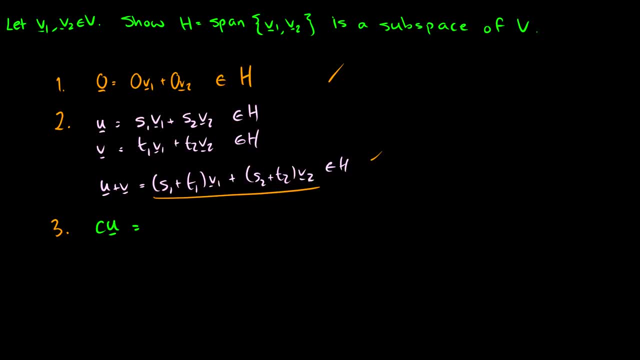 So C times U is going to be C, C times S1V1 plus C times S2V2.. And we know this is in the subspace because this is also in the span. Therefore all three conditions hold. So H, which is the span, V1 and V2, is a subspace of V. 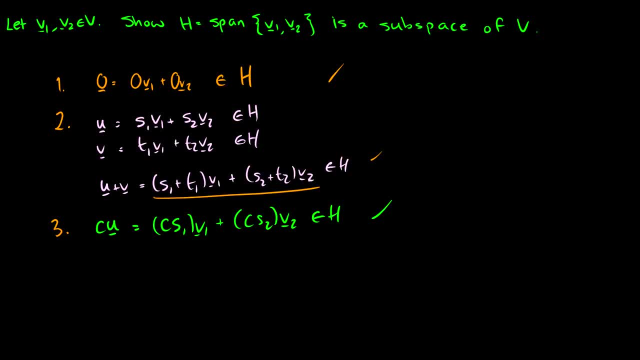 Okay. so if we take the span of V1 through V2 for some vector space, then it's going to be a subspace And we can generalize. So if we have vectors V1 through VP in our vector space, then the span of V1 through VP is going to be a subspace of V. 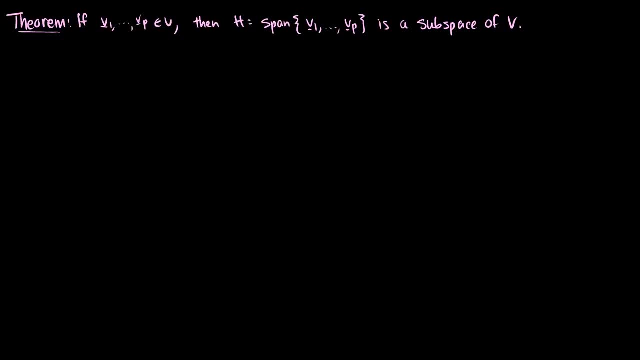 So, again, this is just an extension of what we did before, So we have to show our three conditions. So for the first one, we can show that: okay, well, 0 is going to be 0V1 plus 0V2, all the way up to 0VP. 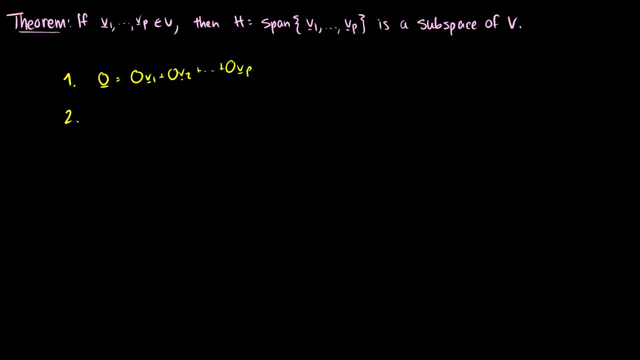 So that's going to be fine. For number two, we did two vectors which went from V1 to V2, and then we had another V1, V2.. So we can do the same thing here. We can take U, we can take V, we can do S1V1 all the way up to SPVP. 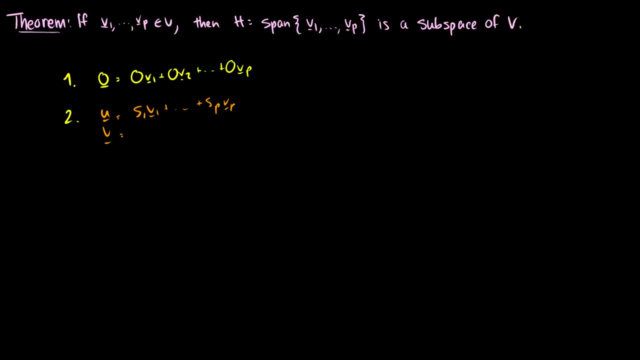 And then for the V vector, maybe we should call it W, And we have T1V1 all the way up to TPVP, And these are just the same steps as previously. But we can see we can extend the result from the previous question and we can extend to this theorem. 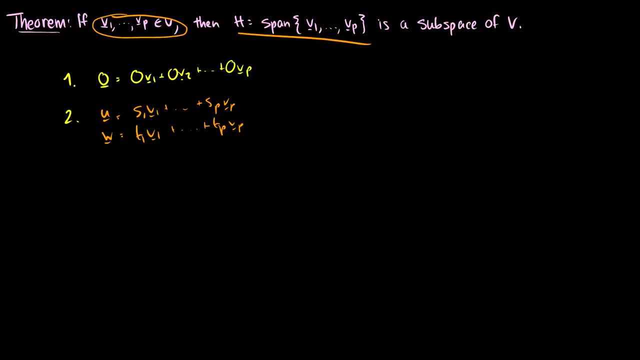 So the H is the span is always going to be a subspace as long as the vectors V1 through VP are in the vector space. So again the same thing for three. it just extends on the previous exercise. I won't do it because all we're doing is, instead of going to V2, we're going to VP. 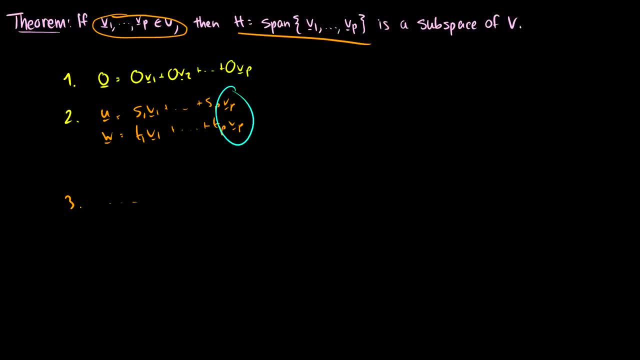 So we just make the addition a little bit longer And it's the same proof. So this is same as last. Okay, so let's move on. Here's a question that you may see in your textbook that looks a little bit more confusing. 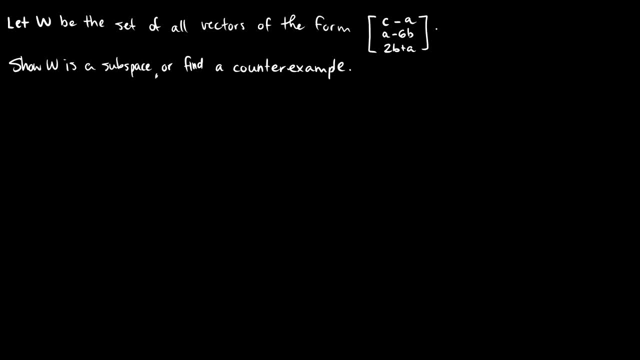 So I say, okay, let W be the set of all vectors of the form, And I have C minus A, A minus 6B, 2P plus A And I want to show that this W here is a subspace. or find a counterexample. 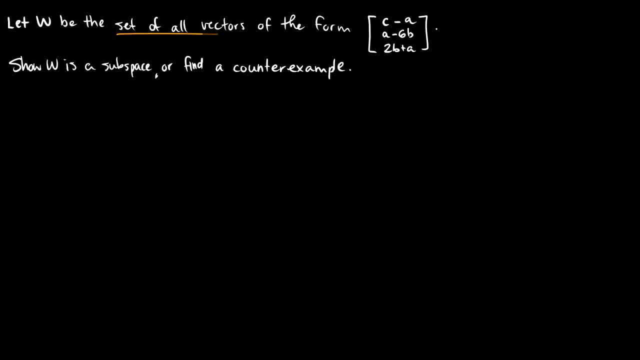 So So W is the set of all vectors of this form. So we just did two things with spans. So maybe we should reduce this to a span of something. Maybe we can get a few vectors here in a span and we can show that this is a subspace. 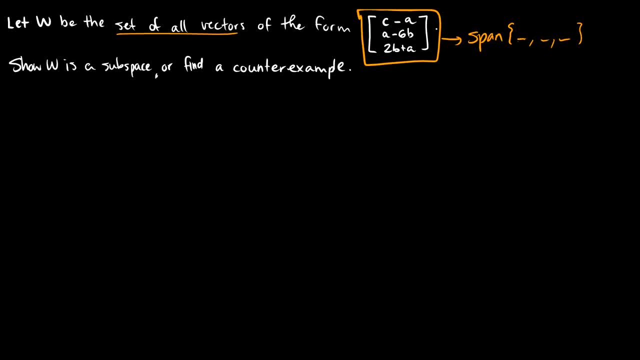 Okay, I should say: show: W is a subspace of V, where V is the vector space containing three entries. So we can say this is a subspace Or three or something like that. But for the sake of this question it's not necessary. 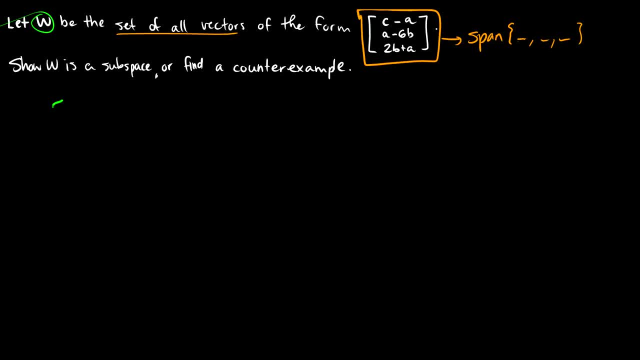 Okay, so we have C minus A, A minus 6B and 2B plus A. So we want to make this a span of something So we can separate this. So what we can do is we can maybe take A times something and then we can add B. 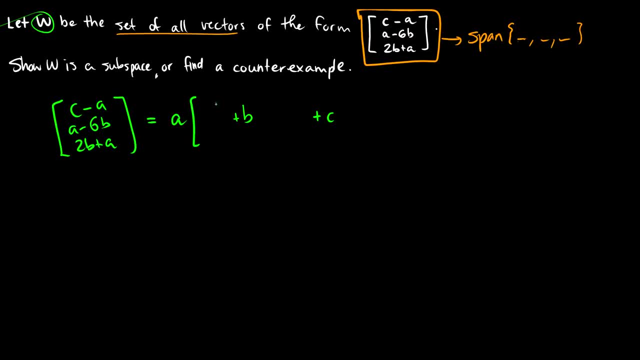 B times something, and then we can add C times something, and then we'll get vectors here. So if we take this form, well, this looks like a span, right? So this is kind of like saying S1V1 plus S2V2 plus S3V3.. 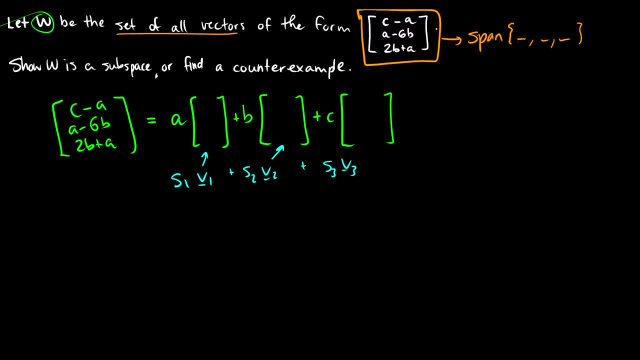 And then we have our V1,, V2, and V3 here. So what are these going to be? Well, we can rearrange, We can rearrange, We can rearrange this to make this a little bit easier to see. 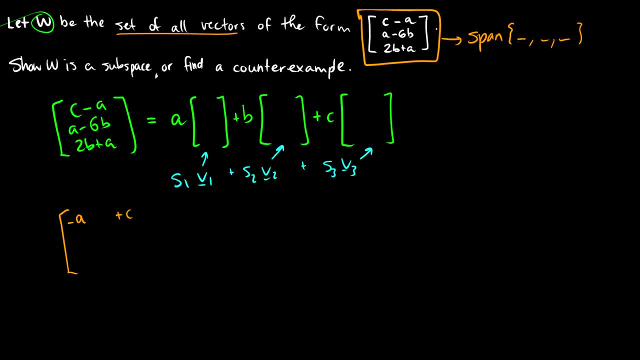 So we have minus A plus C in the first row, We have A minus 6B in the second row And we have A plus 2B in the third row. So we can break this down. So if we take a look at the first column, we have negative A, A, A. 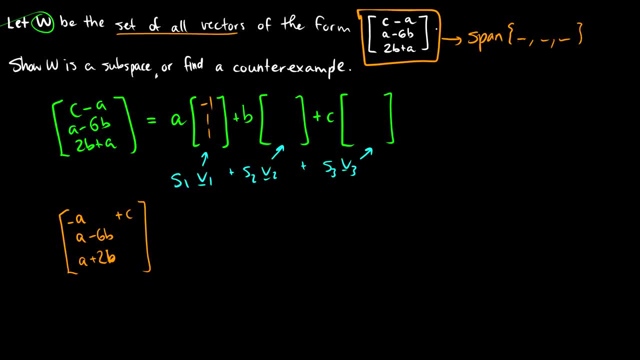 So this will be negative 1, 1 if we factor A out. For the second column, if we factor the B out, we're going to get 0,, negative 6, and 2.. And in the third column, if we factor 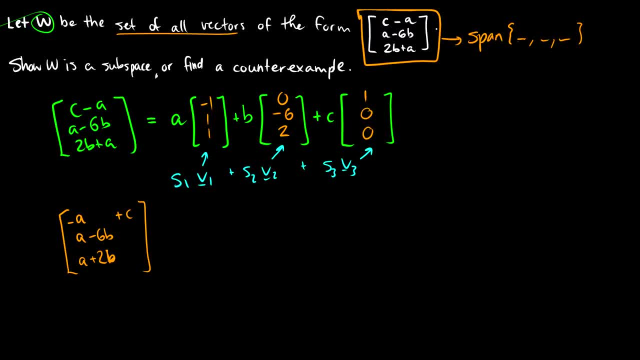 the C out, we're going to get 1, 0, 0.. So we can see now that this is just equivalent to the span of these three vectors, which is negative 1, 1.. That looks like a number there. 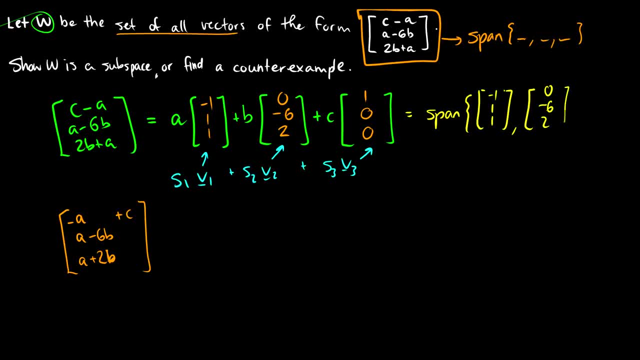 Negative 1, 1, 0, negative 6, 2, and 1, 0, 0. So we know that the span is going to be negative 1, 1, 0, 0. So it's going to be part of, or it's going to be, a subspace. 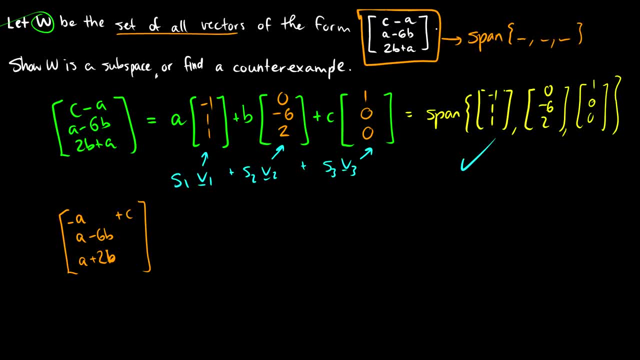 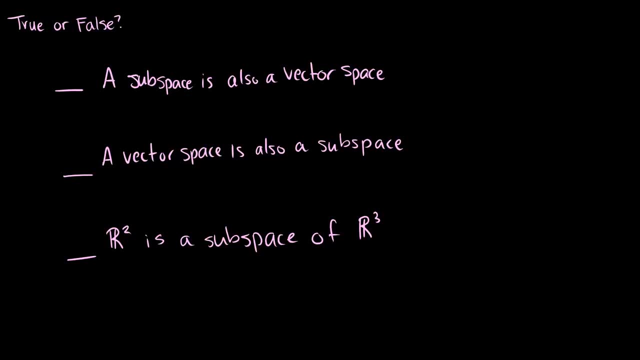 So there we go, We found it. So that is an example question. Now I also have some true or false questions, because when you get to this abstract notion of subspaces and vector spaces, it's good to have a grasp on what we're actually saying here. 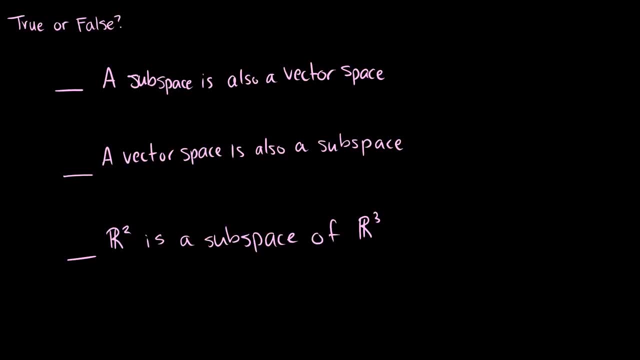 So here's some true or false questions. Question one: a subspace is also a vector space. Well, a vector space space has 10 axioms. a subspace has three main axioms that we have to satisfy. So the subspace, 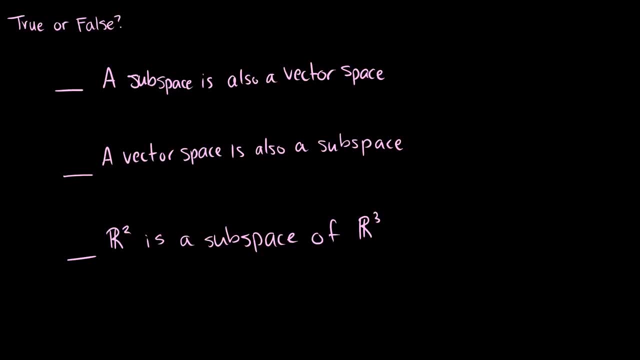 has close under addition, close under scalar multiplication and zero is in the set. But all of these vectors that we're taking are from a vector space, so they're going to satisfy the 10 axioms. Therefore, a subspace is going to be a vector space because we can get access to all. 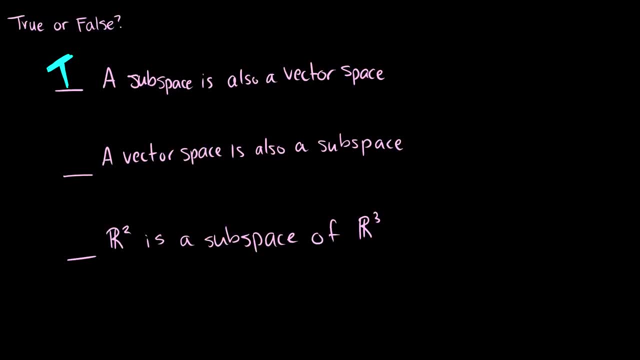 10 of those axioms just from the vectors or the elements that we took from the vector space. Okay, so two: a vector space is also a subspace. This one is also going to be true. and why is this? Well, I should say a subspace g is a subspace of g, So every vector space is a subspace. 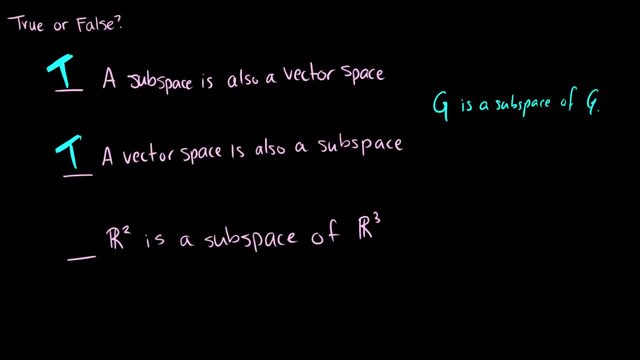 of g. So every vector space is a subspace of g. So every vector space is a subspace of g. Now, this is just like the subset relationship. Of course a is going to be a subset of a if we do set theory, So g is going to be a subspace of g. They satisfy the same criteria, So a vector space. 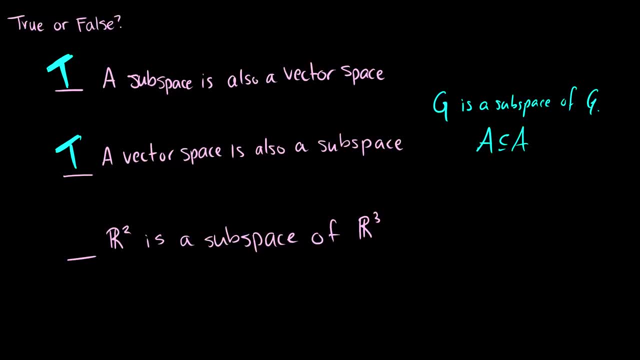 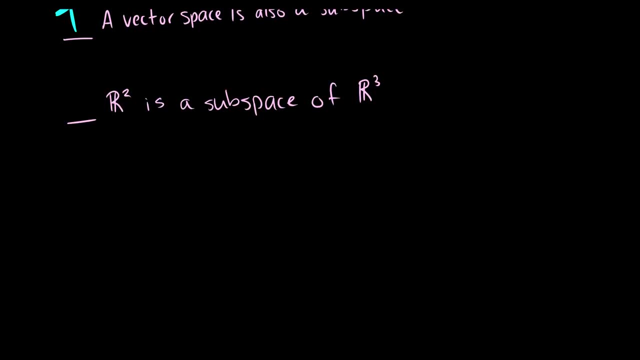 is also going to be a subspace of itself. Last question: R2 is a subspace of R3.. Okay, so here's where you might get tripped up If you're thinking visually, and you might be thinking visually. so we have x1,, x2, and x3.